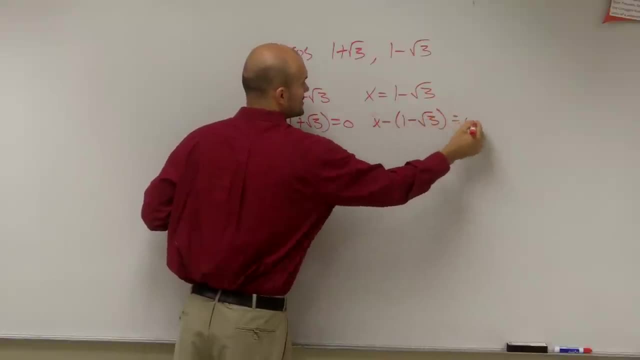 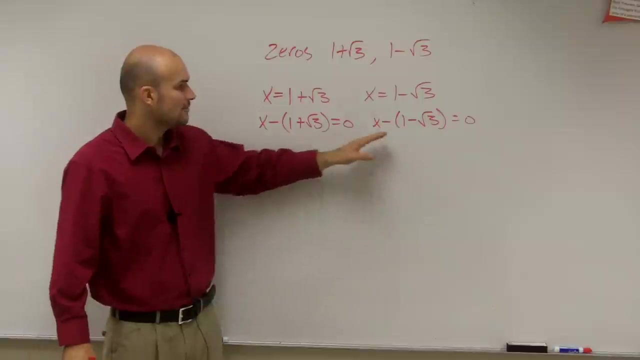 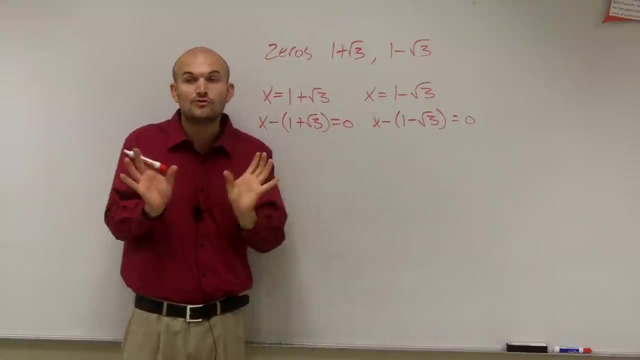 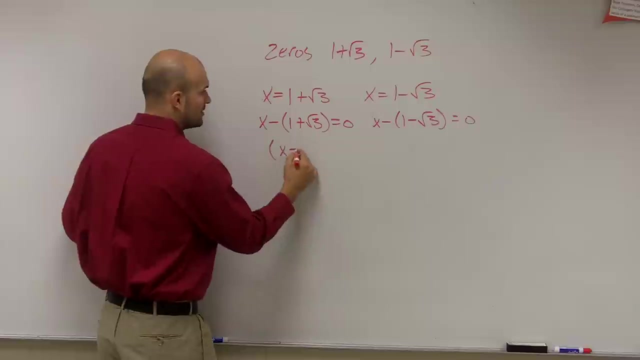 minus one, minus square root of three equals zero. Is everybody following me so far? If not, you can raise your hand. It's totally cool, Okay, The next thing: how we got to this point. remember when we set. why did we set them equal to zero? Because of the zero product property. The zero product property said we had two factors that multiplied to equal zero. So what I had is I had: this times, this equals zero. So that's exactly what I'm going to write. 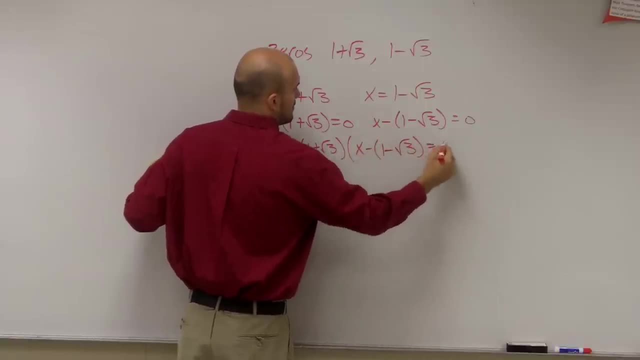 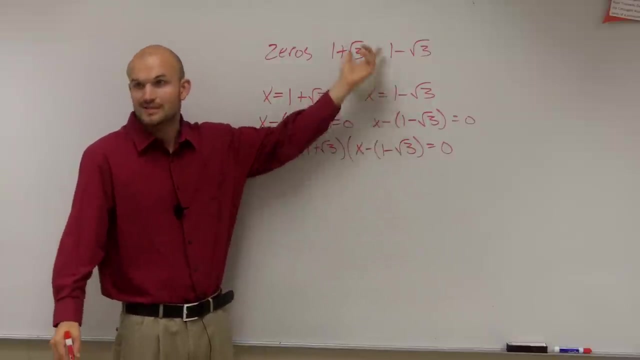 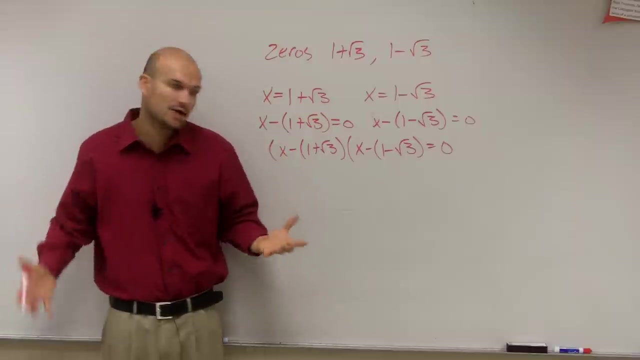 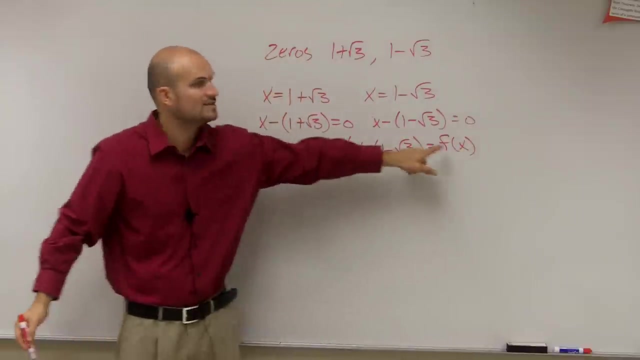 Okay, Right, Remember we had zero product property. You set them both equal to zero and then you solve for x and you get your solutions, you get your zeros. So now I'm just working my way backwards. So now I have two factors and I need to find, figure out the polynomial. So I'm not saying them equal to zero anymore. Now what I want to do is I'm going to call it f of x. When I multiply these out, I want to see what f of x is. And that's what we're trying to get: the polynomial. So here's where it gets a little confusing. 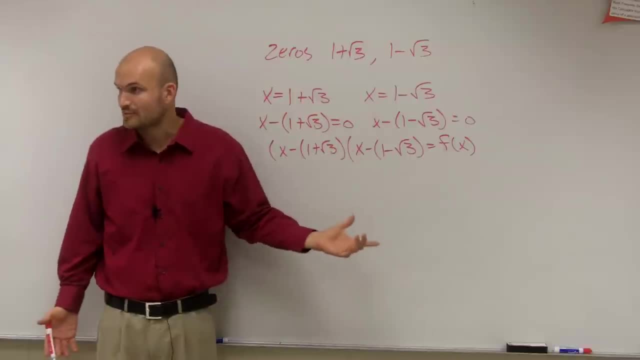 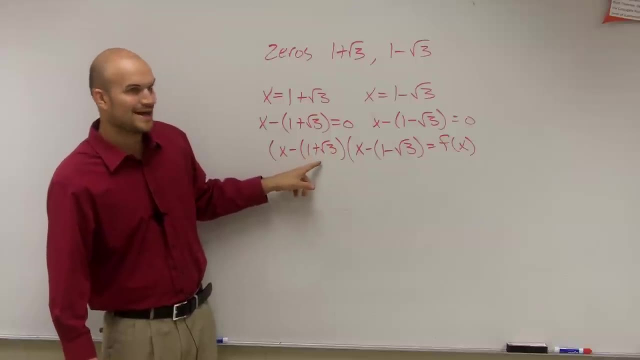 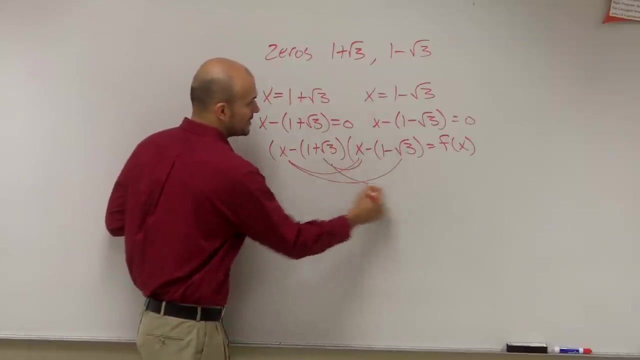 This looks pretty confusing. It's not as easy as your typical FOIL: right First, outer inner last. This is like your last term is a binomial, So this can get pretty confusing. If you're going to try to do the first right, Then the outer inner last, Try to do FOIL with this. You could get a little confused. However, if you're very, if you're very detailed, you can get through it. It's not bad. But I'll show you a little trick. One thing we can do is use the. 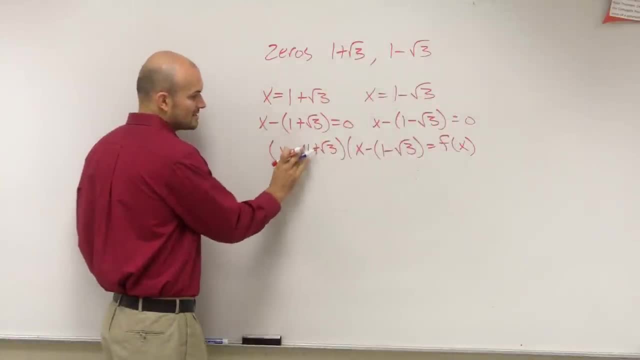 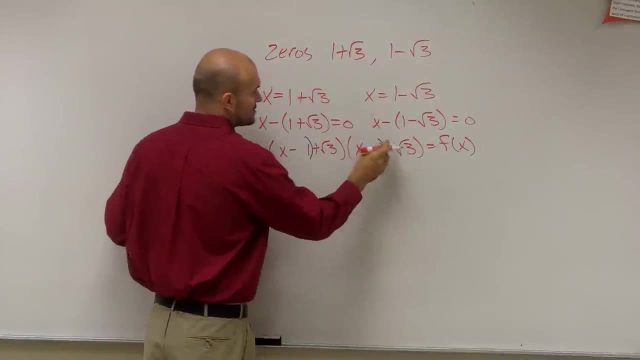 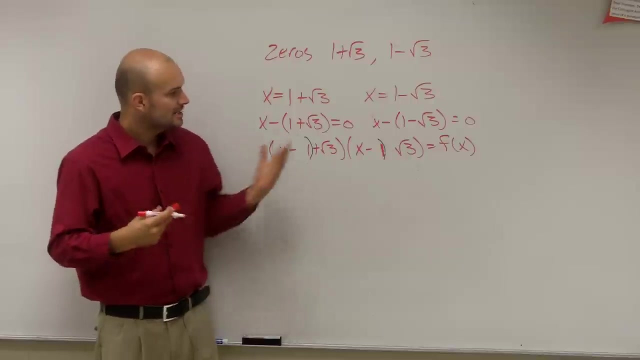 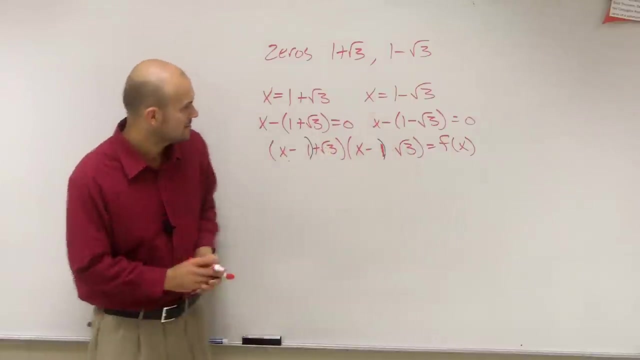 associative property. And what I'm going to do is I'm going to rewrite my parentheses to include, instead of the last two terms as a binomial, I'm going to write the first two terms as a binomial, And the reason why I wanted to do that is because the first two terms, when I write them as a binomial, are exactly the same, And now the last two terms- that's supposed to be a minus- the last two terms are exactly the same. 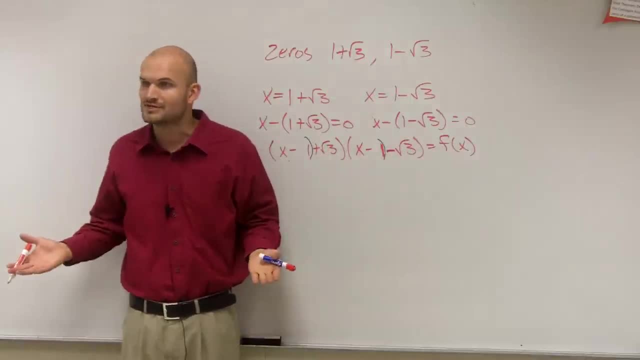 But I have to do something else: have a difference of signs. Does anybody remember when you have the first two terms the same, the last two terms the same and a difference of signs, what would we call that? Anybody Squares? 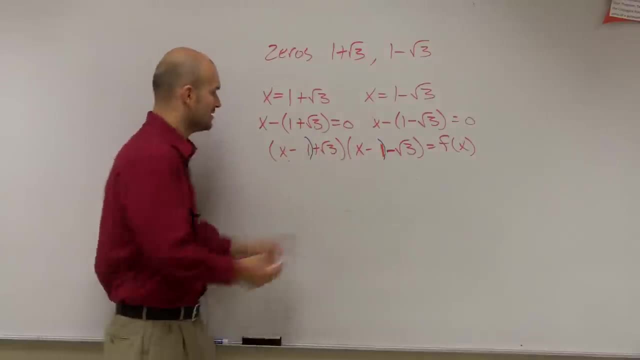 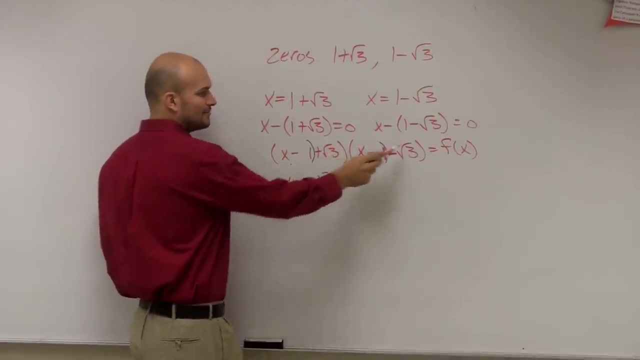 Difference of squares right, Because these two are going to multiply to give me a square number, x plus 1.. So x minus 1 times x minus 1 squared, And then square root of 3 times negative, square root of 3. 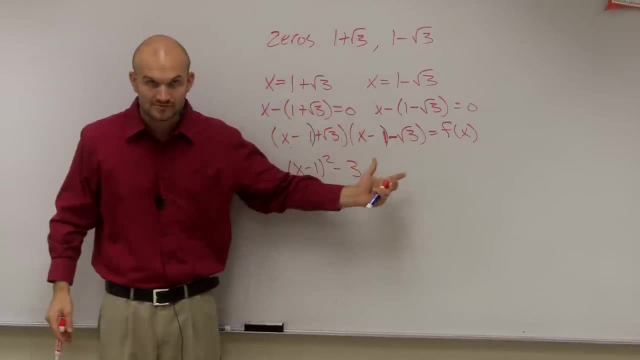 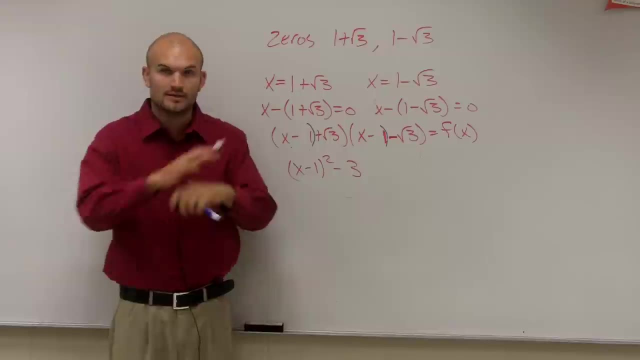 is a negative 3.. I couldn't multiply the middle terms, ladies and gentlemen, And you have to. If you want to follow the rules of FOIL, do it, But what you'll notice is the middle terms cancel out. So I'm just applying the rules of difference of two squares. 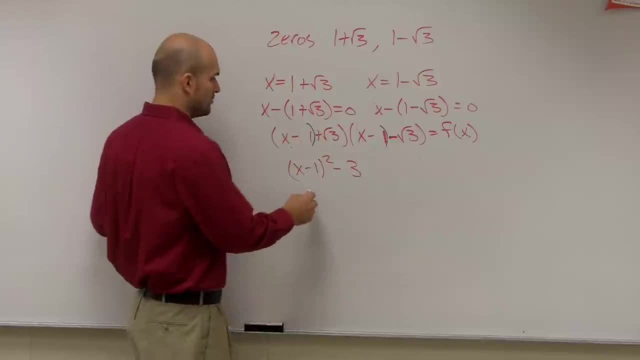 Now x minus 1 squared is going to provide me with a perfect square trinomial That equals f of x. So here we get x squared minus 2x plus 1 minus 3 equals f of x. I'll write the f of x first. 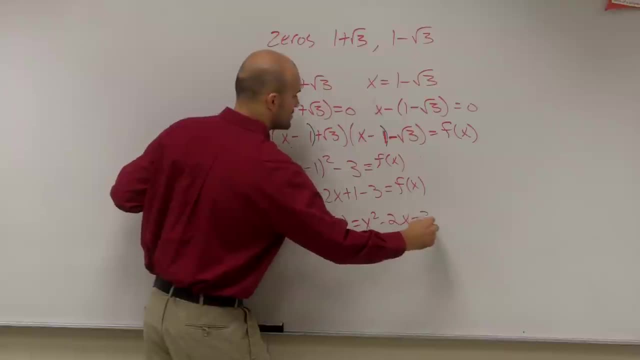 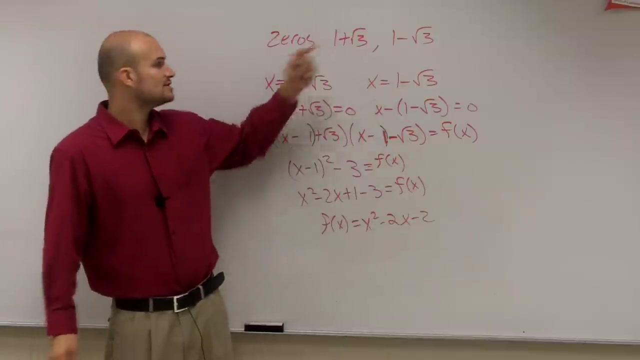 f of x is my function equals x squared minus 2x minus 2.. So therefore, when I have a function x squared minus 2x minus 2, it will include the zeros 1 plus square root of 3 and 1 minus square root of 3.. 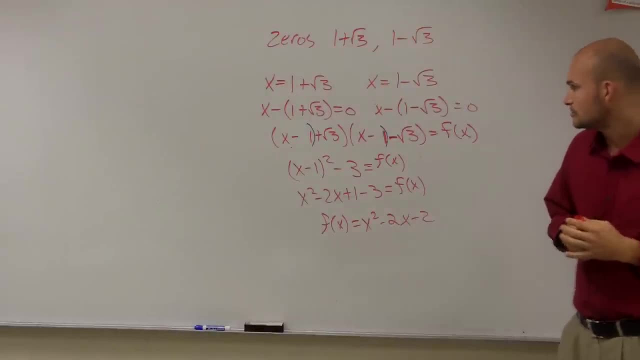 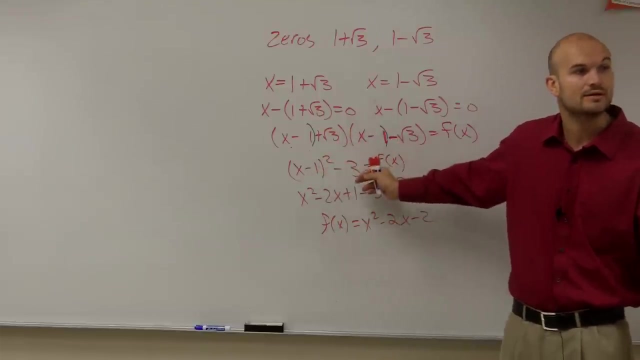 Yes, Why didn't you distribute the negative 3?? Why didn't I distribute the negative 3? You mean here? Yeah, Well, because, remember, it's minus 3.. So it's not being multiplied by negative 3.. It's minus 3.. 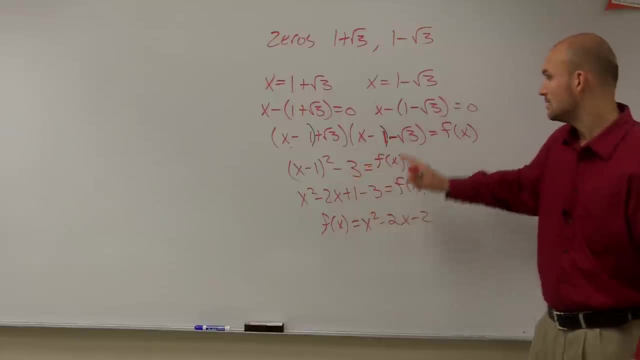 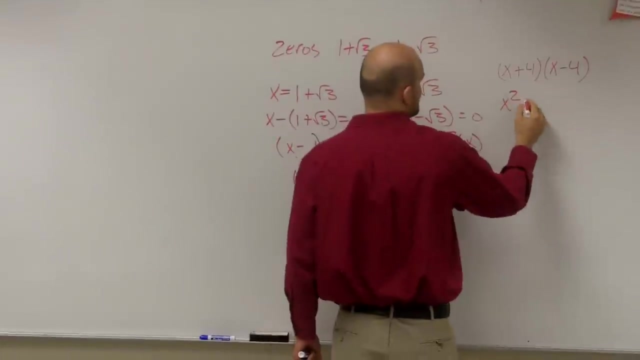 That's why I didn't distribute it. Does that make sense? Remember? it's like: What's the difference? Well, remember, I had something like this: x plus 4 times x minus 4.. So when you multiply this out, you get x squared minus 16.. 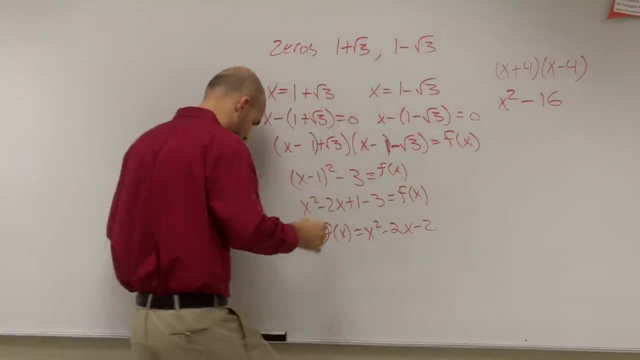 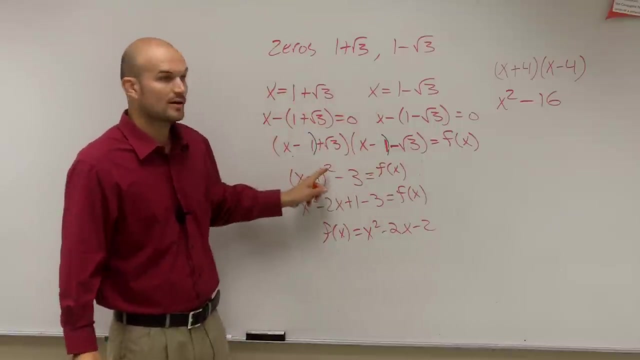 You don't distribute like the negative 16.. It's x squared minus 16.. The only difference was: I'm getting tangled around. The only difference is: now I have it's just a binomial that's being multiplied. Instead of x squared, it's x minus 1 squared minus 3.. 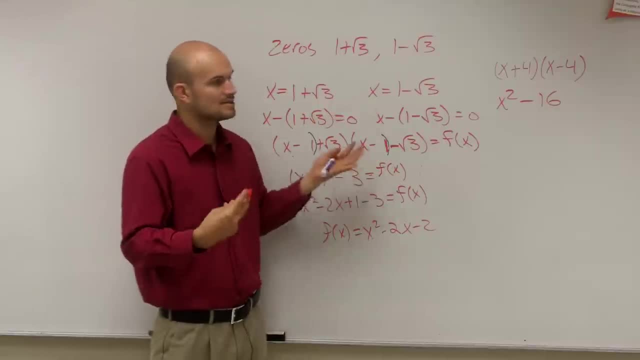 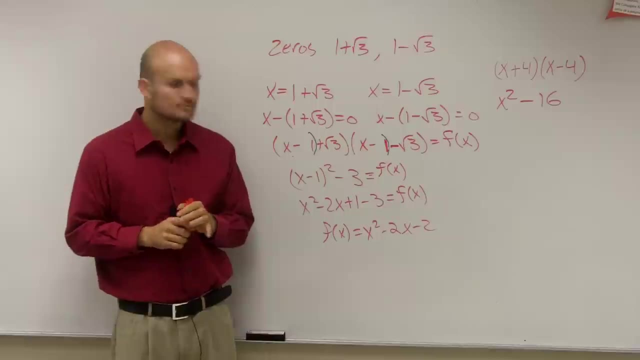 Does that kind of see it? I know it's a little bit. this looks a lot more different than that, but it's the same kind of process. Cool, Yes. So since the how do you call it? Radical? Since they're opposites, they equal negative 3?. 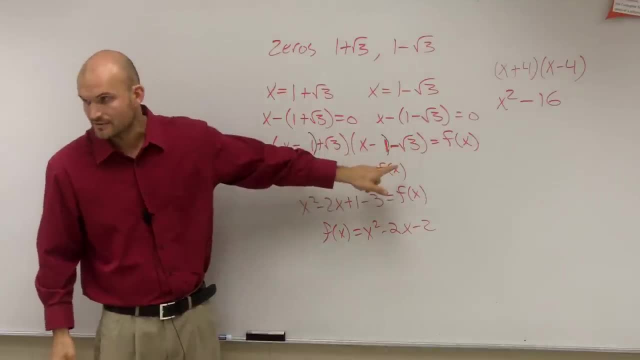 Since the yeah, Yes, That's a positive and that's a negative, So it's always negative. Yeah, positive times, a negative will give you a negative Right. And then square root of 3 times square root of 3 gives you 3.. 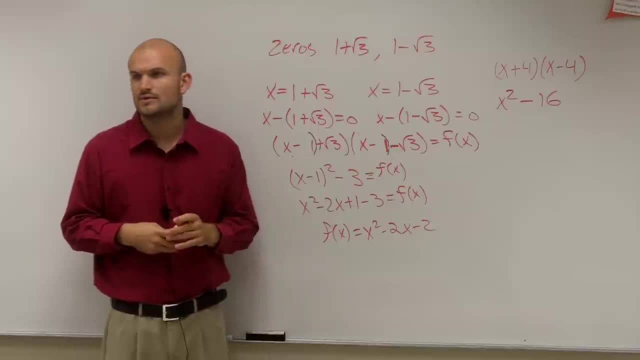 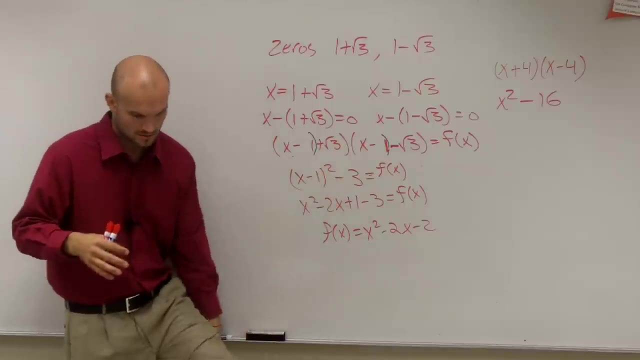 Which other one do I know of 60? 61.. 61. Oh, but can you have a 60 to negative? I'll see what I can do, But anybody have questions on this? 60? Oh, I thought you said 62.. Right, OK.